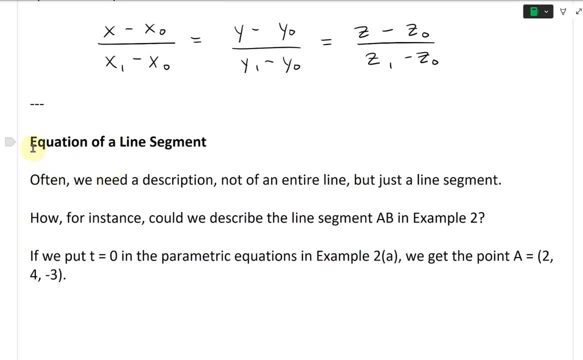 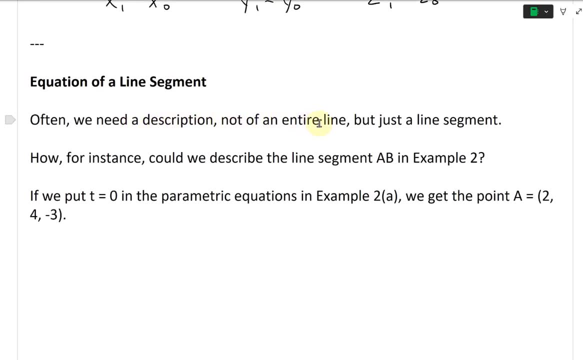 All right, now let's continue further and look at the equation of a line segment as opposed to just a full, infinite line. So often we need a description not of an entire line, but just a line segment, or but of just a line segment. 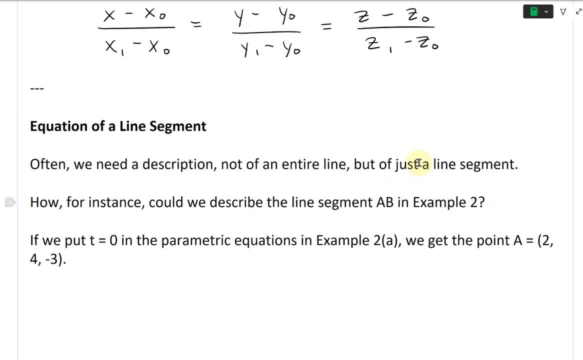 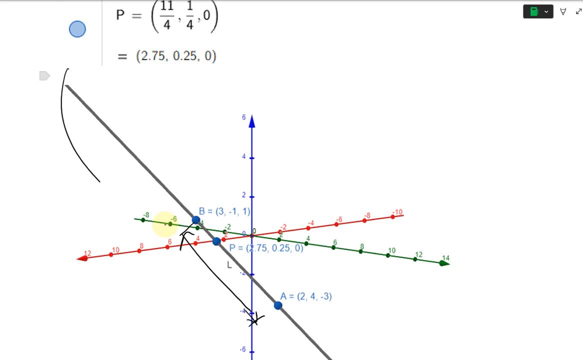 How, for instance, could we describe the line segment AB in example 2?? So how could we describe this right here, from here to here, as opposed to drawing this entire line like that? So we just want the line from A to B like that, so that line segment. 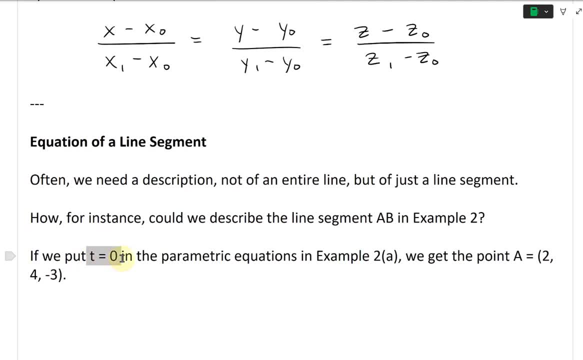 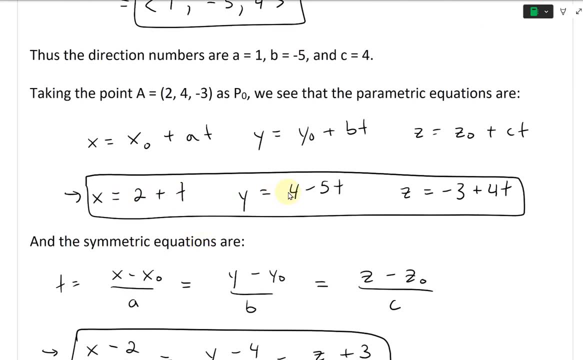 All right, so going further. so if we put T equals 0 in the parametric equations of example 2A, so those are right here, this parametric equation. So if we put 0, here we're just going to get X, we're just going to get the yeah, X naught and then Y naught. 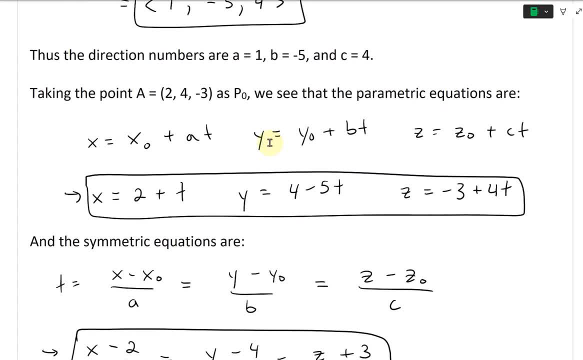 Z naught, And then the next one. we could just put 1, and then we're going to get actually interesting results. So let's take a look right here. So if we put it in, we get the point. well, 2,, 4, negative, 3.. 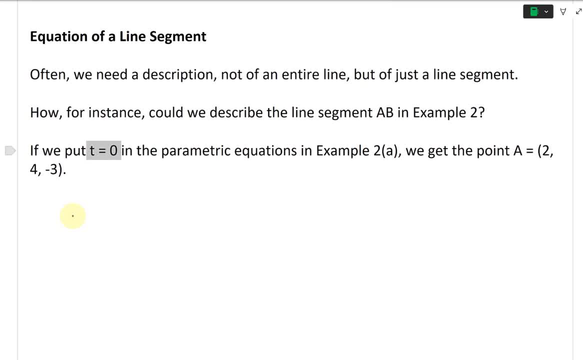 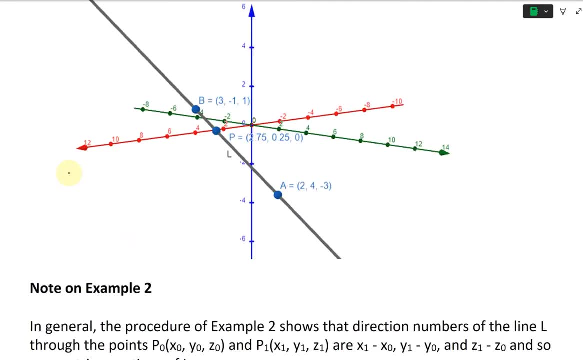 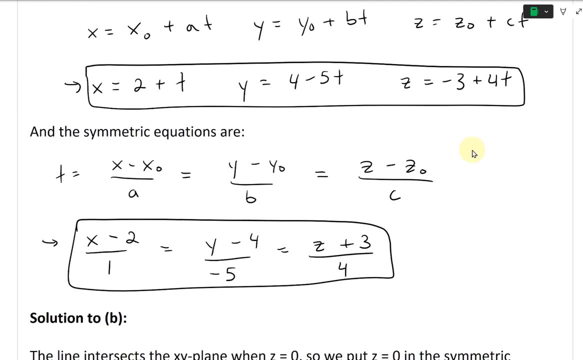 That's just a point A and you could see that Again this is just X equals 2, and then let's just put that line again: plus. I believe this was 2 plus T. So going back here, this is yeah, 2 plus T, then 4 minus 5T and this is negative: 3 plus 4T. 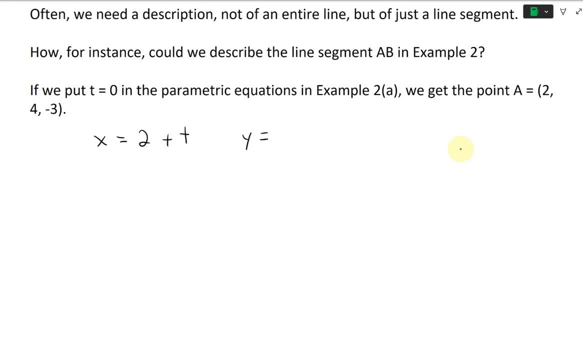 All right. And then Y is equal to 4 minus 5T and Z is equal to negative 3 plus 4T, like that. And then when you plug in 0, well, we get. so let's write this here for completeness: 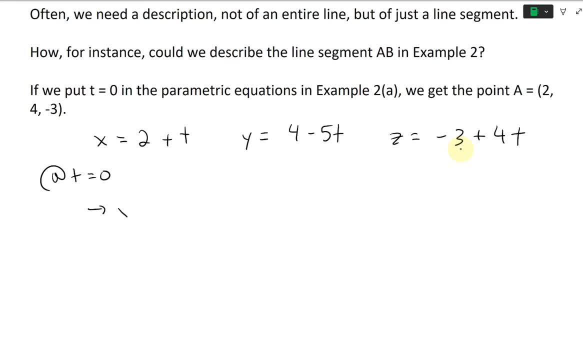 At T equals to 0,, everything vanishes. We're just going to be left with X equals to 2, Y is equal to 4, and then Z is equal to negative 3, which is again this point. right here is just our A. 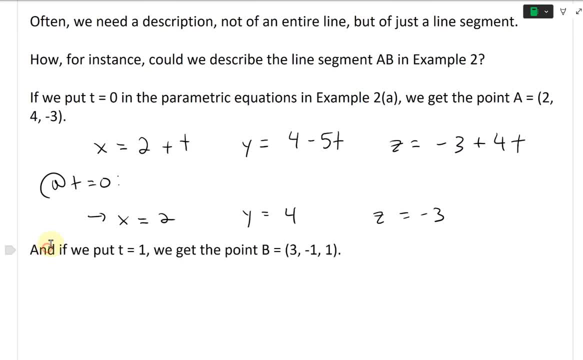 A is a negative, 2, 4, 3, like that. And then if we put T equals 1, we get the point B, because this just becomes yeah, 1, and that's just going to be the coordinates that you're subtracting, the coordinates of. 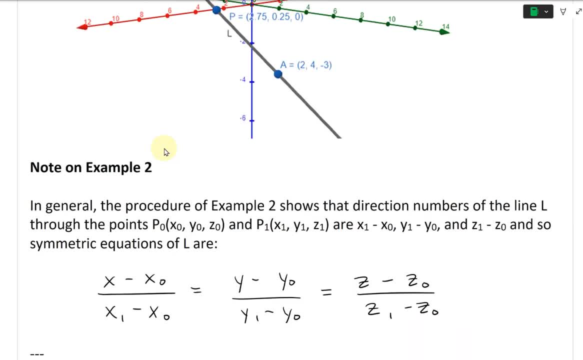 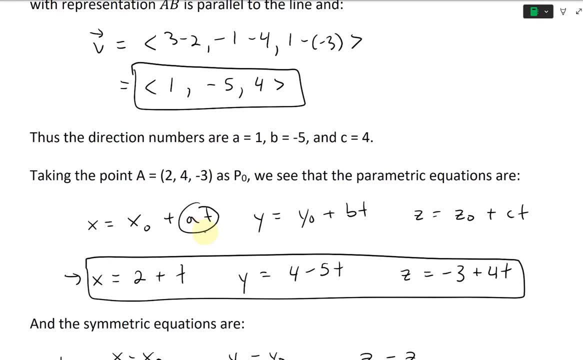 Actually no, this is a direction number. So if we remember these equations- yeah, just a top word up here- These equations right here that we got, for example, this was AT and then A was 1, where 1 was 3 minus 2.. 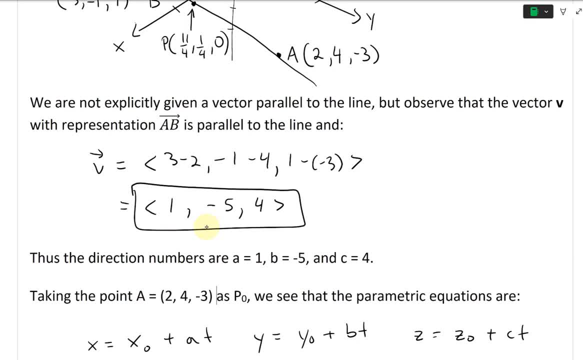 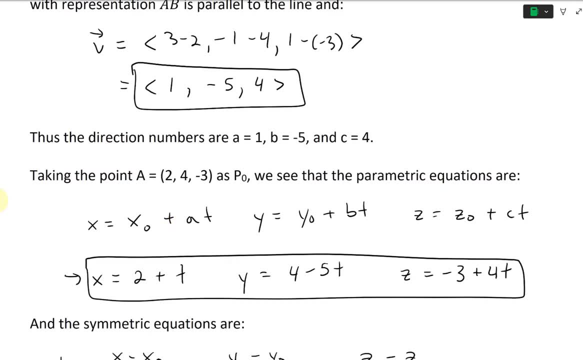 2. So, in other words, in this first example we have, yeah, this 3 minus 2, this is our X1.. You can consider that as X1.. So we have. we'll have it right over here. 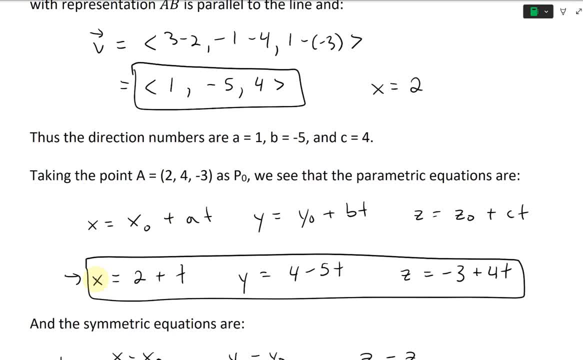 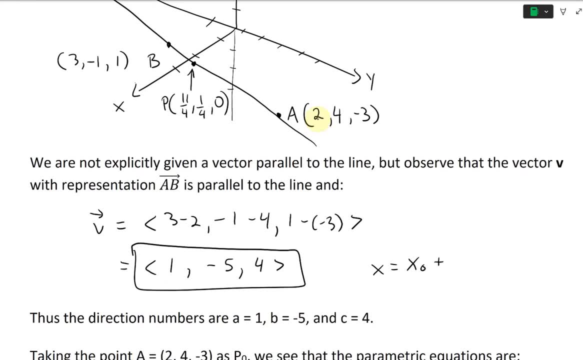 So X. let's write it here. X equals to 2.. And then the 2 right here is just our X naught. This equals X naught plus, and then the A value, which was going to be X1 minus X naught T. 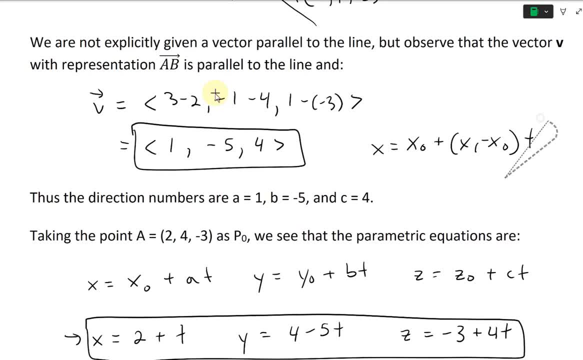 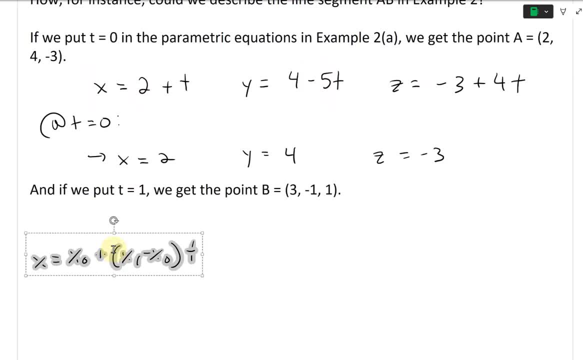 So then, if this is equal to So, if this is equal to So, if this is equal to- and now we that we have this written, I'm gonna copy and paste this and then let's put it down here. yeah, we get here and if we look at it, if you plug in, T equals to. 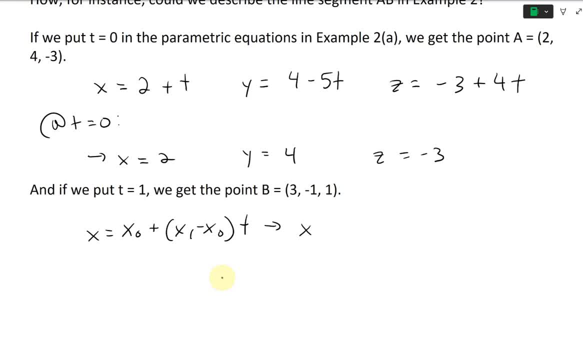 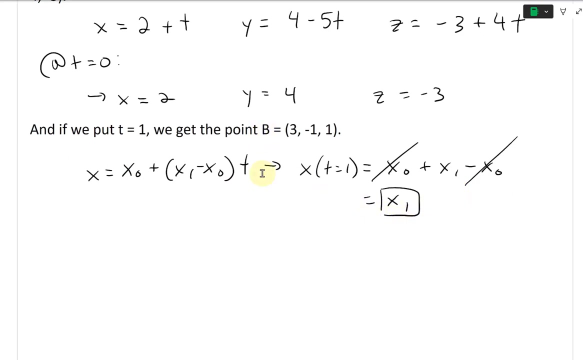 1, we're gonna get X. X at T equals to 1 is equal to X naught, then it's gonna be plus X 1 minus X naught, and then these just cancel. so the left, so it's X 1. so in other words, and then do the same thing for Y and Z, we get the point B. so 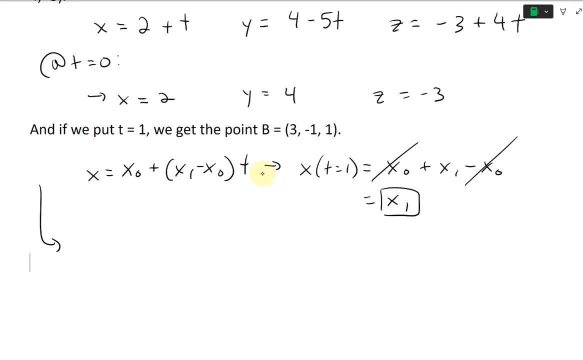 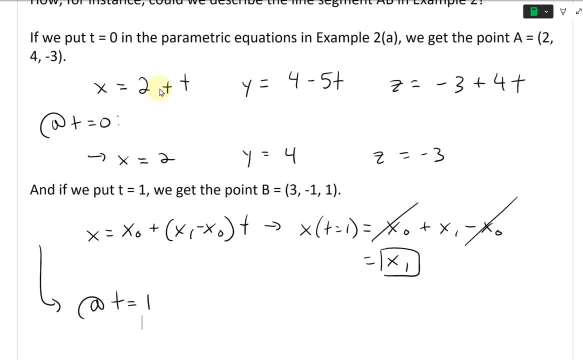 in other words, here at T equals to 1 for our, for our scenario, we get T equals to 1. plug in 1 here, so 2 plus 1, 4 minus 5. so right this year. so this is gonna be, yeah, it's gonna be 3. 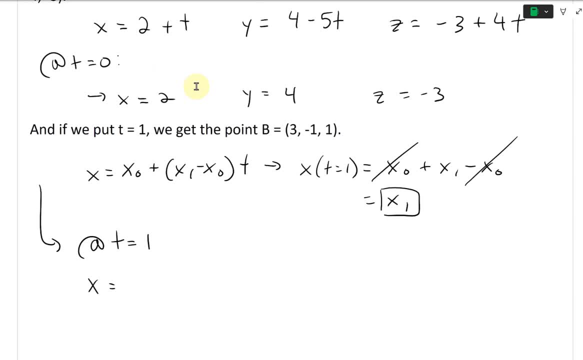 negative: 1 and 1. so you go plug it as in: 2 plus 1. 2 plus 1 is equal to 3, so that's correct. then the next one is: Y is equal to those boxes and this is the correct answer. and the next one is gonna be right here: 4 minus 5 times 1 is 1. 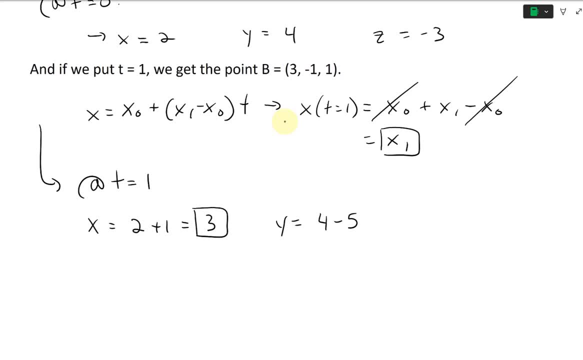 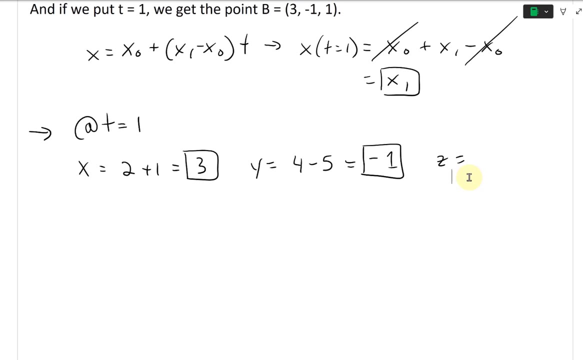 yeah, yeah, 5 times T is a, 5 times T is just one, is negative 5. this equals negative 1, and that is correct. the Zed- is it gonna be equal to zed- equals 2. negative 3 plus 4t, so negative. 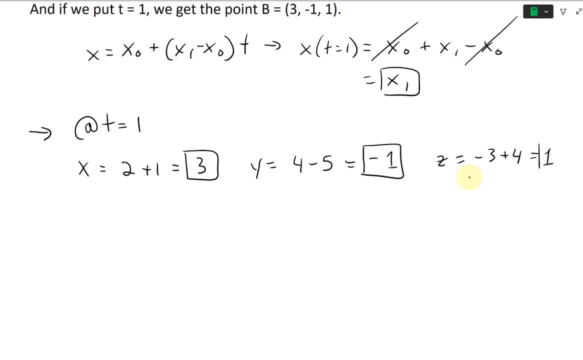 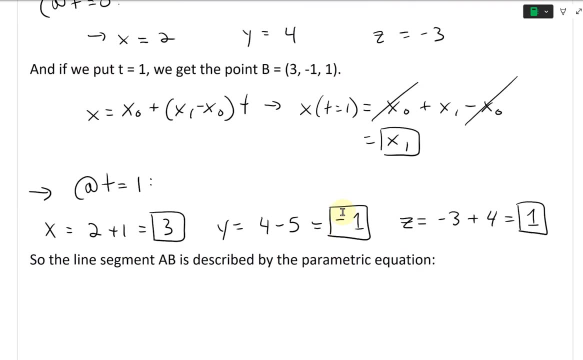 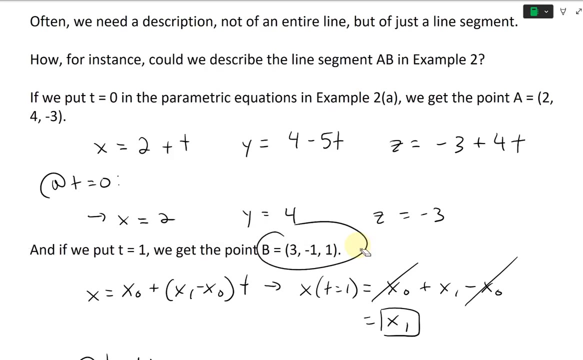 3 plus 4, that just equals to 1. so 4 minus 3 is 1. yeah, so the line segment AB is described by the parametric equation because again it ends up- bad be here that T equals to 1. it ends up het B at a. T equals 0, it ends up with ace. 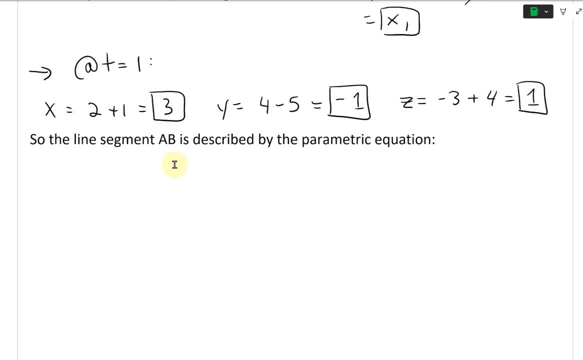 So, in other words, all we need to do is solve it: from t equals 0 to t equals 1.. So, in other words, the equation- I'll write this here: r of t, the line segment. this equals 2.. 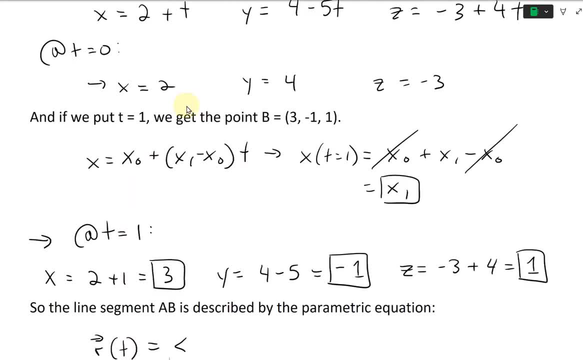 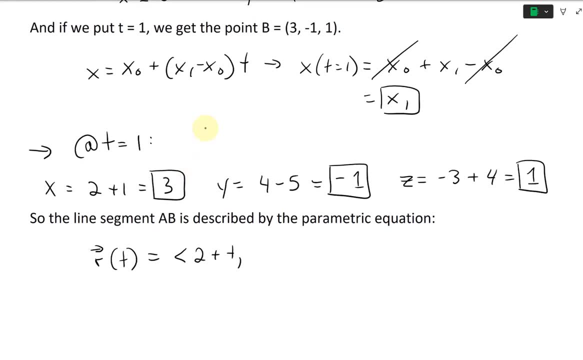 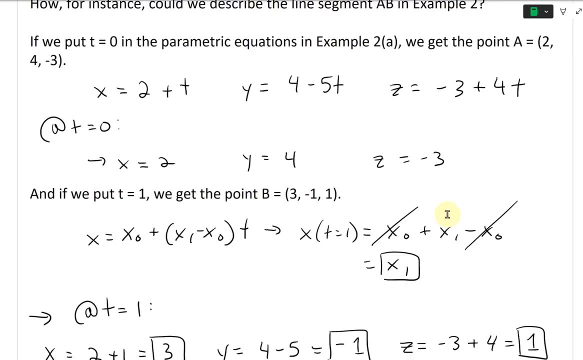 And this is a vector equation form And that is just putting these all together. So this is the parametric equation. So 2 plus t is the x component, And then we have: y is equal to 4 minus 5t, And then we have this negative 3 plus 4t. 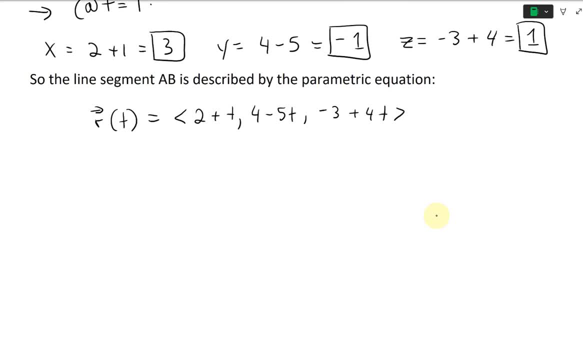 Negative 3 plus 4t- And this is 4t- is less than equal to 1 and greater than equal to 0. So this is the line segment from a to b. Exit this All right. so, going further, let's generalize this. 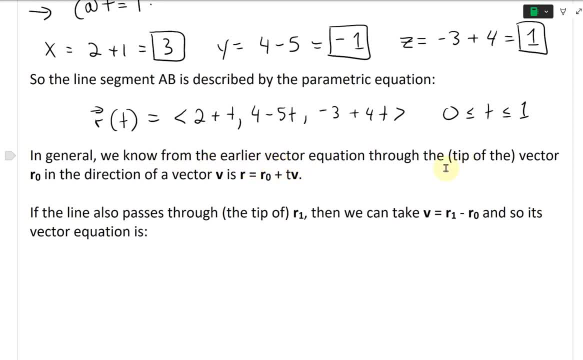 So in general we know from the earlier vector equation: through the tip of the vector r0 in the direction of a vector, v Is r equals 2 r0 plus t times v. That's just the vector equation of a line. So if the line also passes through the tip of r1 vector then we can take v is equal. 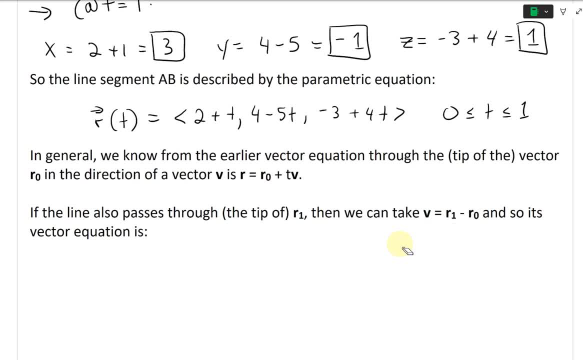 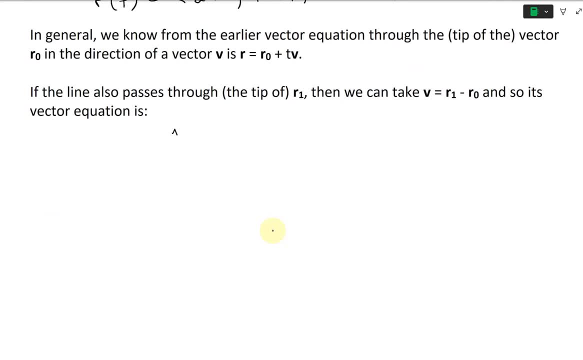 to r1 minus r0, this vector And so its vector equation is- And before I write that, I'm going to actually draw it out just to illustrate this graph- This is going to be Z, actually Like that. So that's our z. 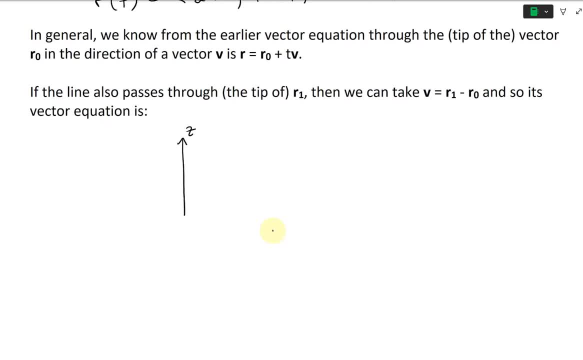 And make this a bit less steep, And then this is going to be our y And this is going to be our x, Like that. So let's say we had a line l like this. Just make it like that. This is our line l. 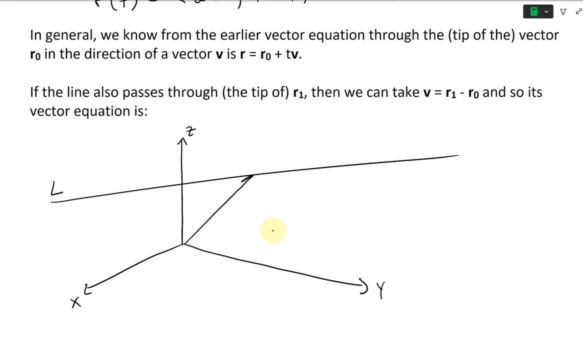 And it has this from the origin. Let's say we have our r, Not vector, So from the tip, here is on the line. And now let's say we had right, here is going to be our r. So let's say this is our r. 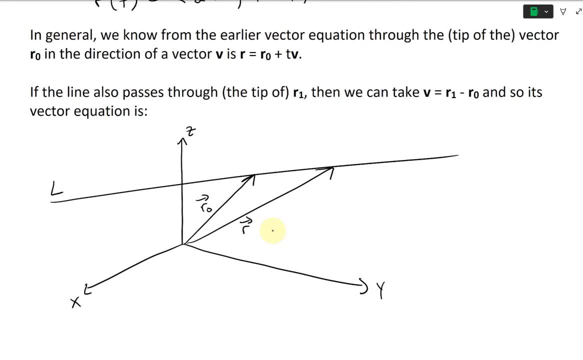 And this is our r vector. It's a vector equation And before we draw the t v, Let's say we had r1 is somewhere here. This is another point on the line is r1. And now We're going to draw this in red. 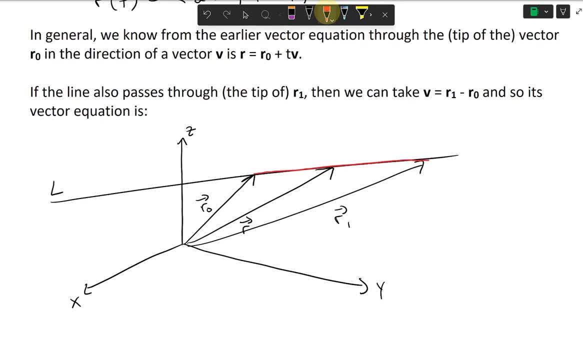 So let's say we had a vector. This is the vector v. This is going to be v, like that. Yeah, this vector goes to like that. And from this vector you'll see that r0 is equal to r. Yeah, this is going to be r0 plus v. 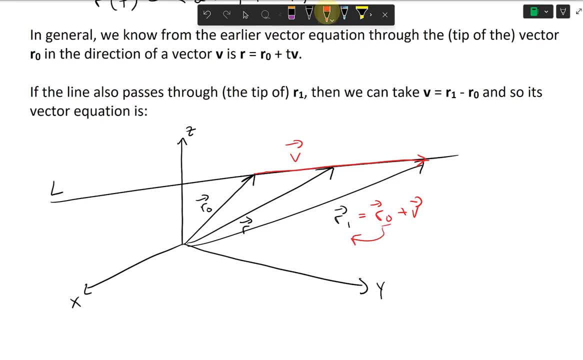 So, in other words, to solve this v, we just move this over to the other side And we subtract it. We get this equation right there And this is the triangle law. like this, r0 plus v is equal to r1, like that. 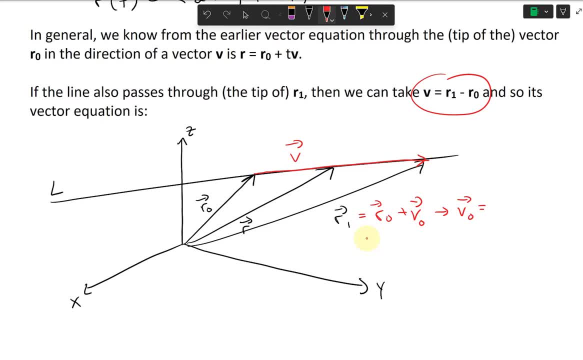 And again, this just means that v is equal to r1 minus r0, like that. And here I just change it to black, felt like that, just to make it easier to see. So anyway, so that's that part, And this is our r. 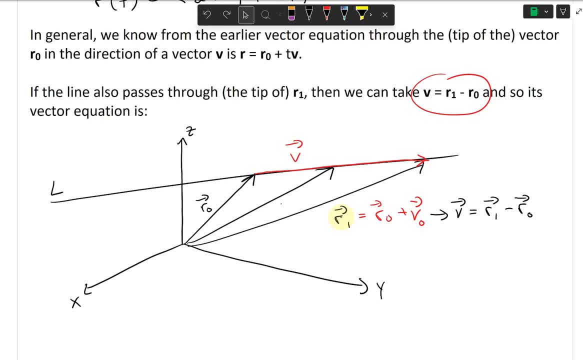 Oops, this is going to be our r. Our r is this one right here, And then the tv is going to be just a scalar times, this v, And that's going to be across here. It's going to be like that, Whoops. 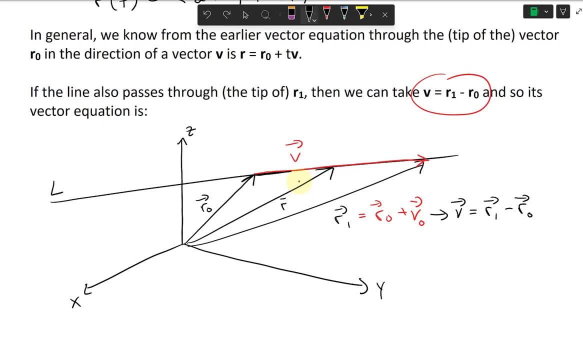 That's just going to be. It's going to be actually. I just want to make this a bit neater, So put the r0 here. This is going to be tv0. Or actually not v0. I mean just v. 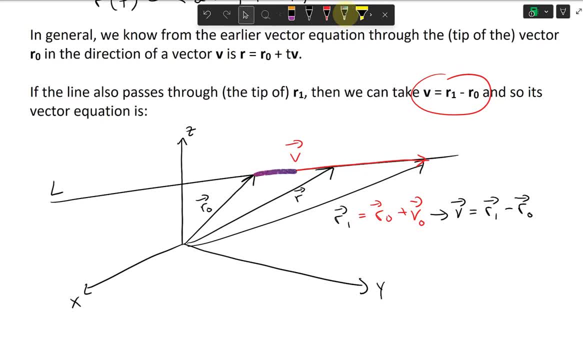 And I'll erase that again. I'm just going to put this in blue. Or this is not blue, This should be blue here, And let's make this in blue, And that's going to be like this. All right, let's draw this again. 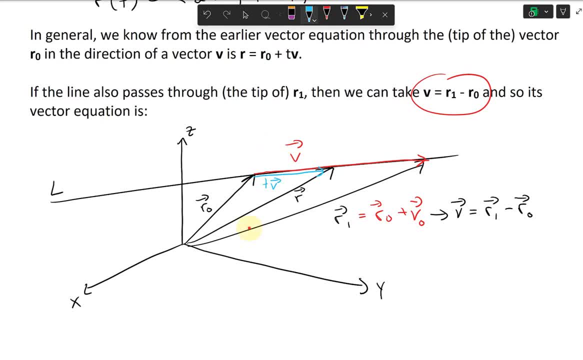 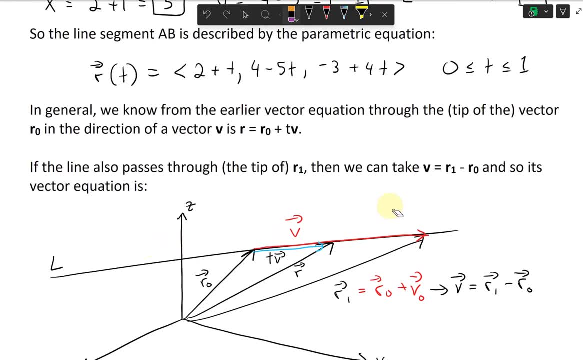 Yeah, so this is going to be tv vector, And here I just made it black so it's easier to see. All right, so that's what we have. So, going back to this, we're going to solve the vector equation. 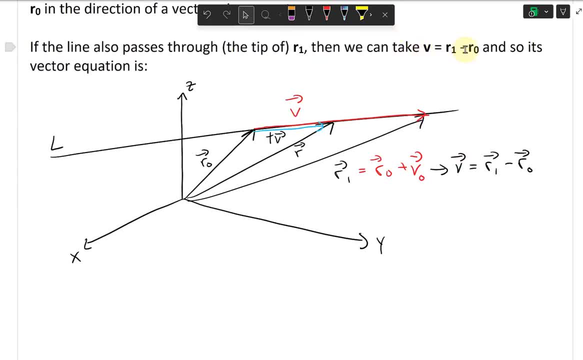 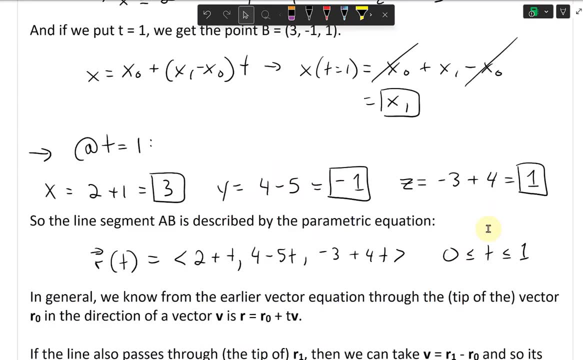 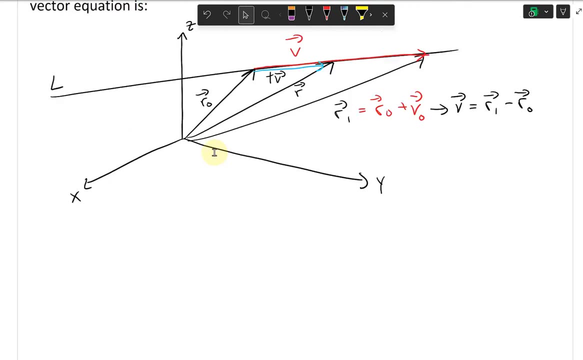 So, using what we know, using this, v equals to r1 minus r0.. Just like this setup that we did for the line segment right here, Yeah, in which we found a difference between a and b in the components and so on. So let's go back here. 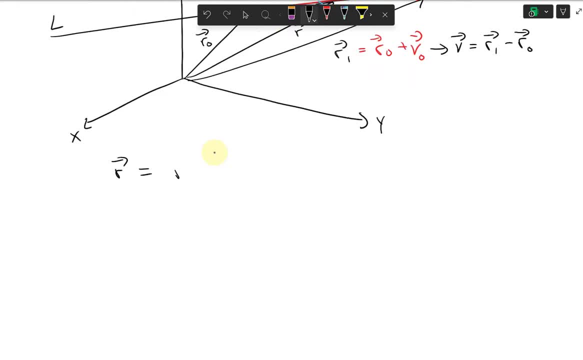 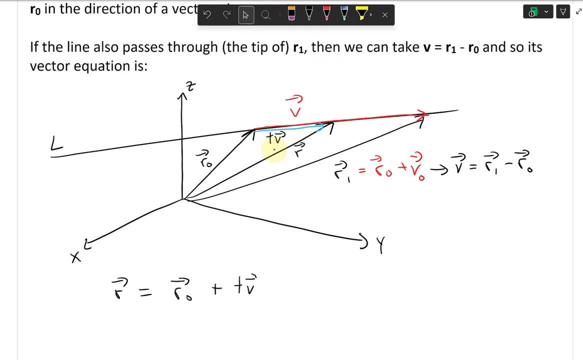 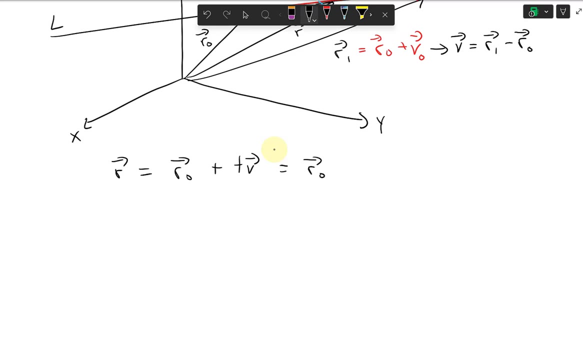 So this is going to be now r vectors equal to, well, r0.. So r0 plus triangle rtv, right there, Tvvector, And this equals to- let's write it all over here: This is going to be r0 plus and then t, then the vector v is equal to this part, right here. 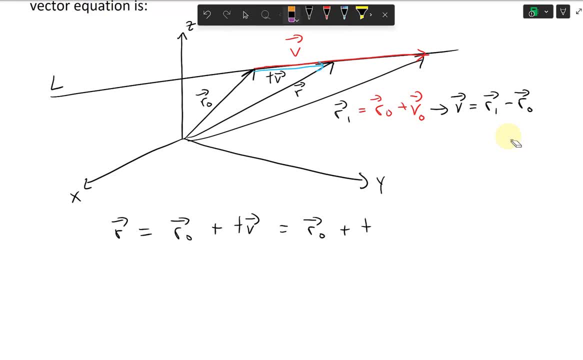 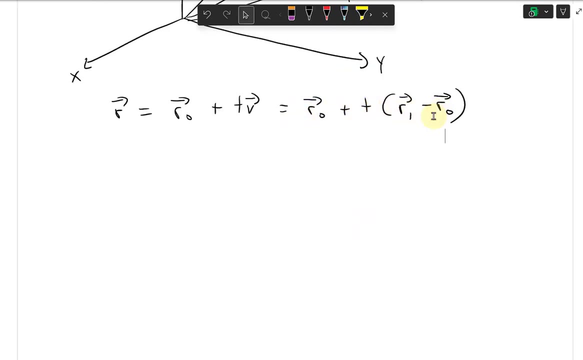 So that equals to this is going to be t times r1 minus r0 vector, And now we can just simplify this out. So multiply this t inside and separate the like terms, And what we get is- I'll write this like this: 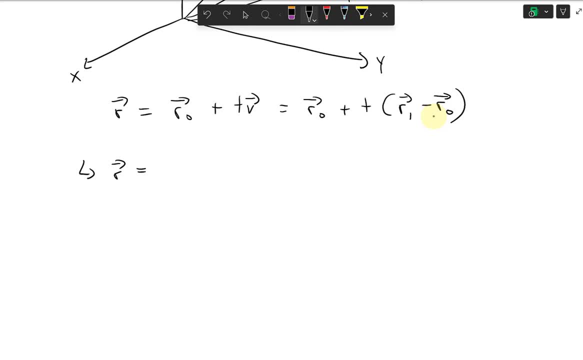 This equals to r0.. I mean r vector, not r0.. This r0 equals to: this is going to be: well, we're going to factor out. Well, let's do this all on completeness. Yeah, let's do it all on completeness. 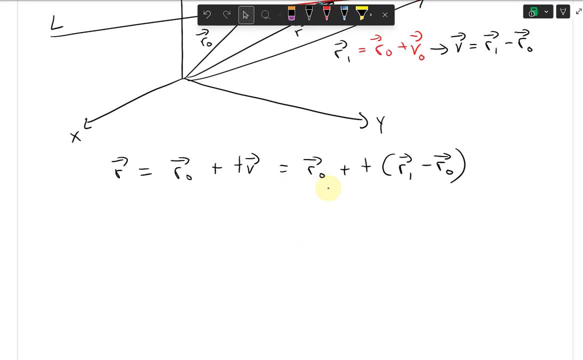 We're going to erase this, We're going to write this all later. So this equals to that. This equals to here: r0 plus tr1, vector Minus tr0.. And now we can separate the factor out, the r0s, the like terms. 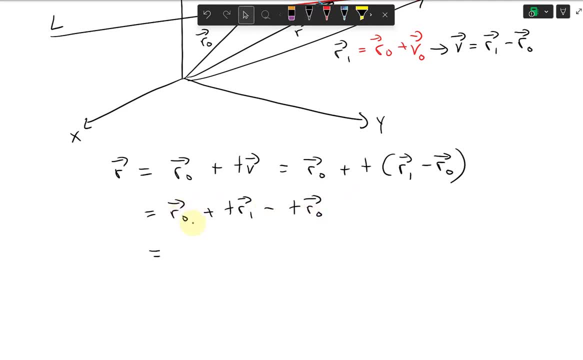 That's going to be, and then you factor out: it's going to be 1.. I'll put it over here, And that's going to be 1 minus t, Like that, And then plus tr1 vector, Like that. 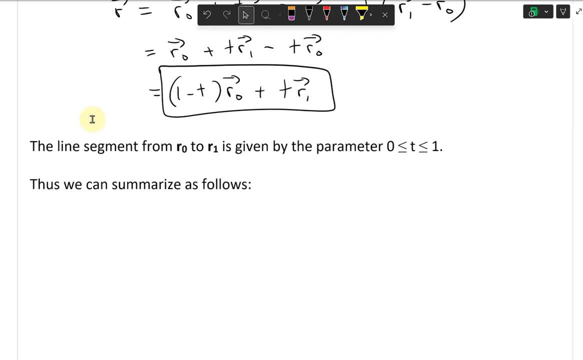 And I'm just going to box this in Like that. And now this setup here. if you look at it, it's the same thing as we had before. So if we put in, If we put in, t equals to 0, this vanishes. 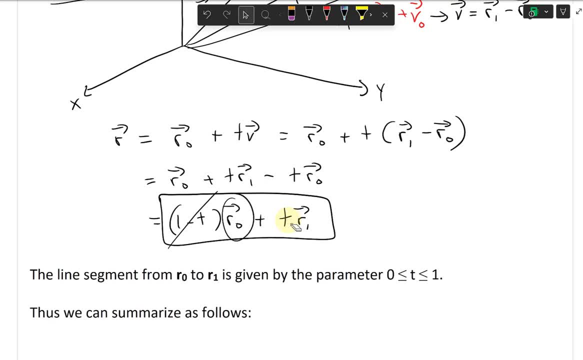 This becomes 1.. So all we're left with is r0.. Likewise, if you put in: t equals to 1, this vanishes. This whole thing vanishes, Yeah, this whole thing vanishes, And this becomes 1.. 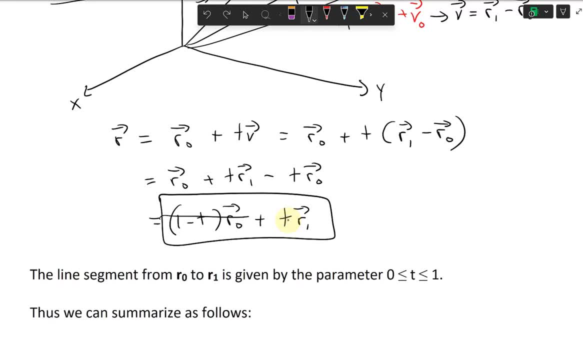 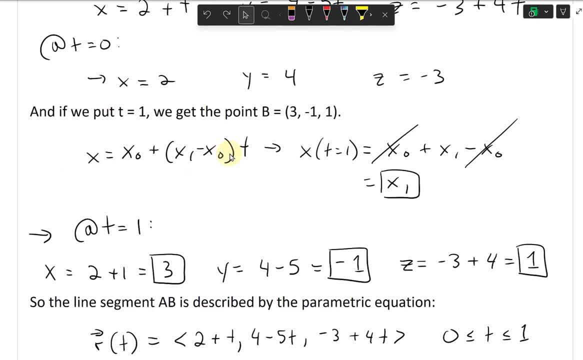 And you're left with r1.. In other words, it's exactly what we had earlier, but in that scalar format I wrote here: So x equals to x0 plus x1 minus x0. Like that t. And then when you plug in, t equals to 1,. 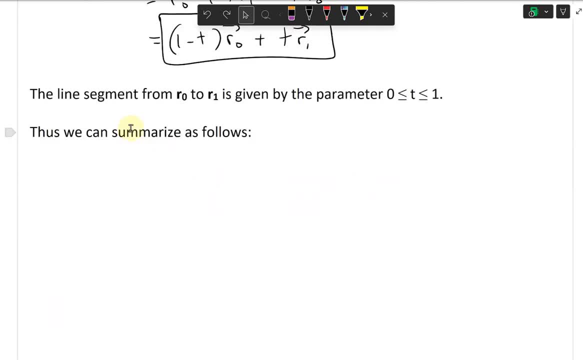 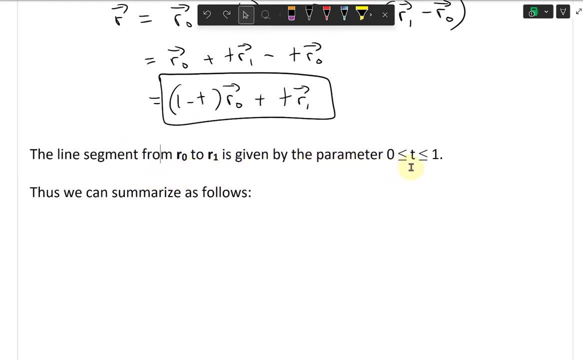 the x0s vanish, They just separate. So it's exactly what we just had, but here I'm writing it in vector form. So the line segment from r0 to r1 is given by the parameter. 0 is less than or equal to t. 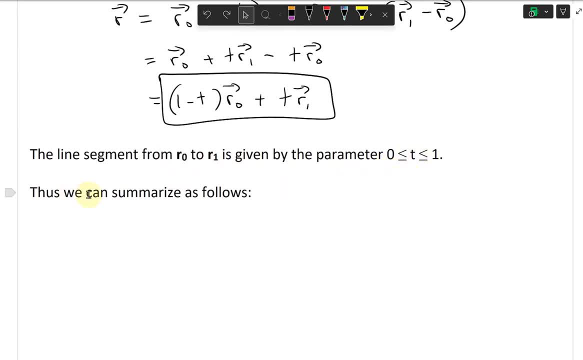 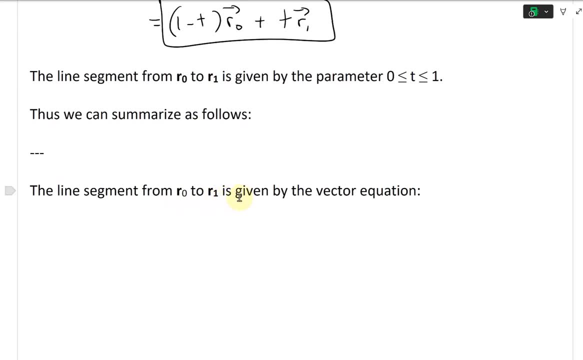 which is less than or equal to 1.. So t is from 0 to 1.. Thus we can summarize as follows: And this summary is right here. So the line segment from r0 to r1 is given by. this should be bold. 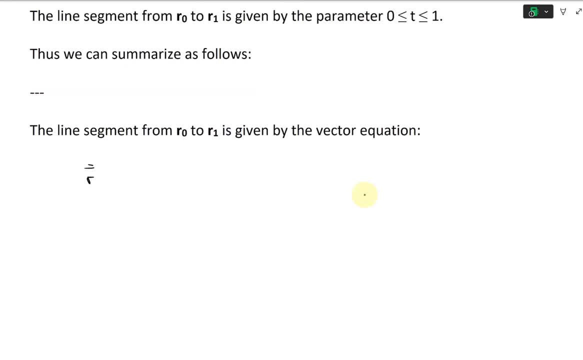 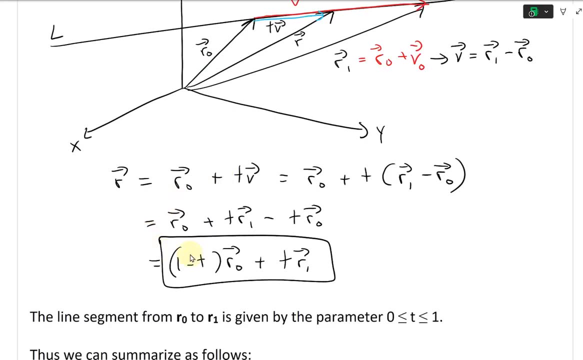 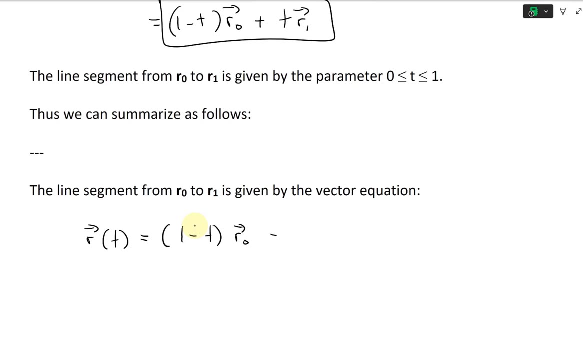 given by the vector equation rt, I mean r of t, So r is a function of t. equals to this right here: 1. 1 minus t r0 and then plus t r1, like that where t is less than or equal to 1,. 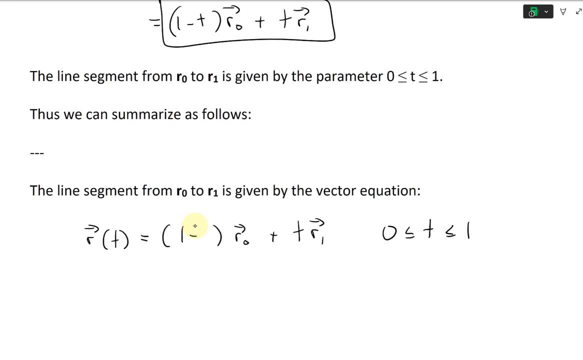 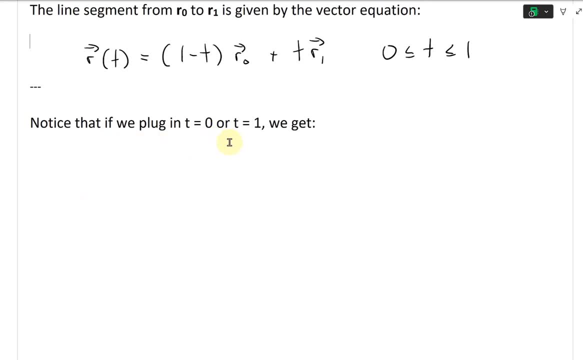 greater than or equal to 0. Like that, All right. And again, as I just alluded, to notice that if we plug in t equals 0 or t equals 1, we get well r of 0, this just equals to. 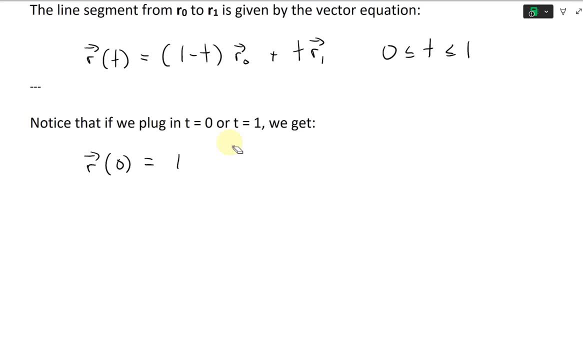 this is going to be 1 times by r0.. Yeah, let's put it all together: 1 minus 0 r0 plus 0 times r1, like that This just becomes. well, this is going to be 1.. 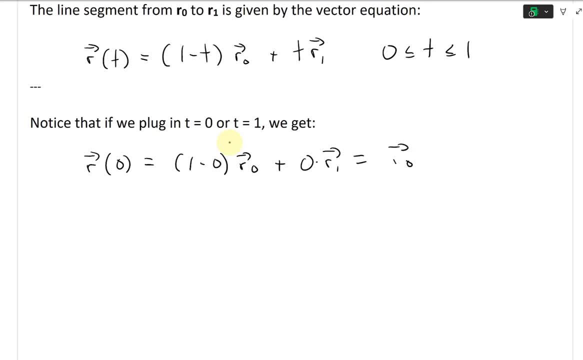 That's going to be r0 vector, like that. In other words, that's where it's going to, that a value Or the starting point on the vector on the line. So then r1, so t equals 1, we get 1 minus 1 r0 plus 1 times by r1.. 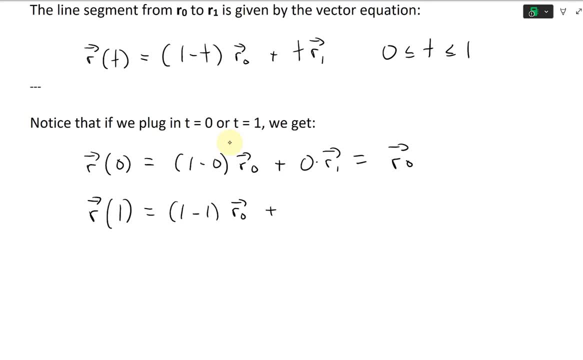 Let's leave that 1 out And this is going to be r1.. This just equals to this vanishes and we're left with r1, like that Box, this box, this, And this one is the vector to that second point on the line.